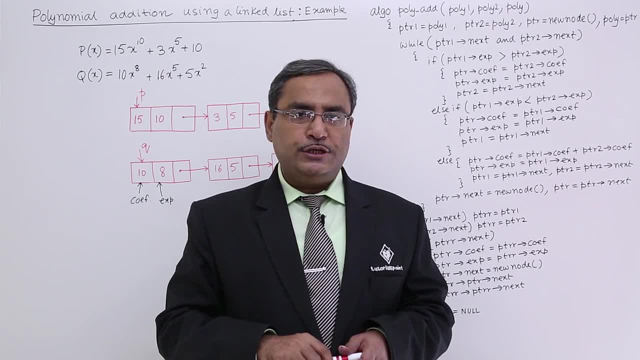 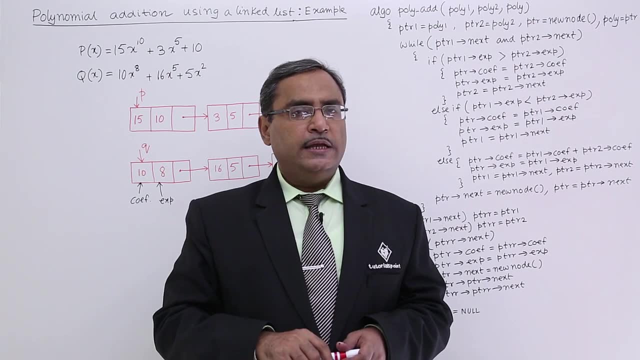 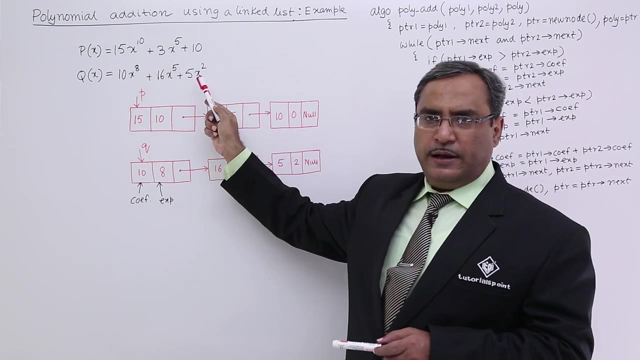 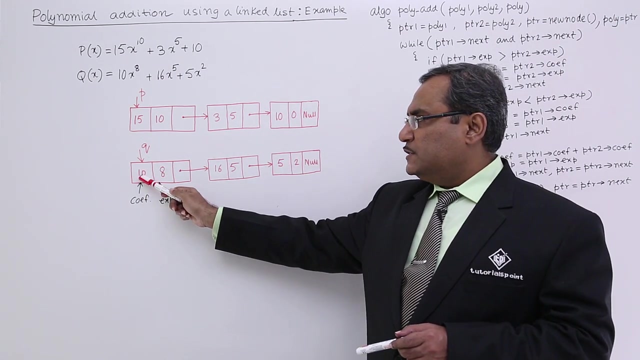 In this session we are discussing polynomial addition. In our earlier session we have discussed how a polynomial can get represented using a linked list. There we have demonstrated that px and qx- two polynomials were given and their respective implementation through linked list we have discussed And the first field is known as a coefficient. the second field is known. 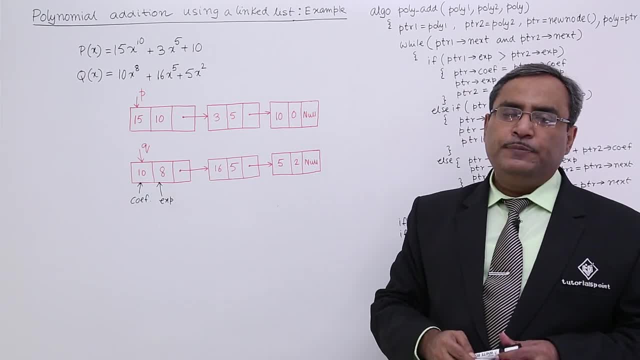 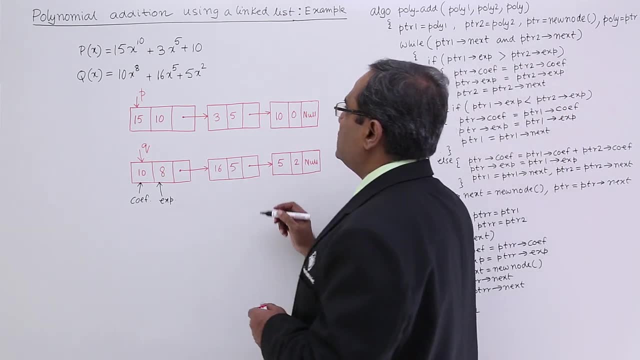 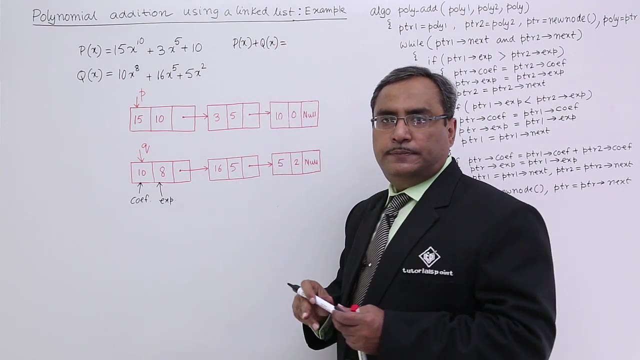 as the exponent, and the third field is known as the link or next field. In this way they got expressed. Now, if I want to perform px plus qx, then what will be the result? We know that at first we should consider that very term. 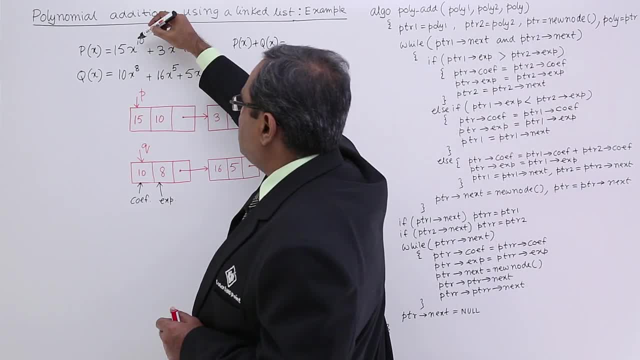 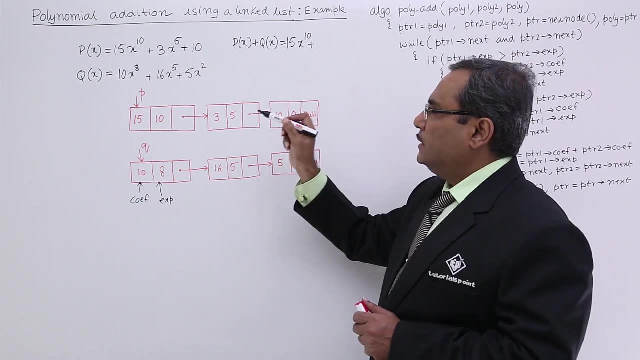 which is having the exponent maximum, which is having the exponent maximum, So it is 10.. So it should be 15.. x to the power of 10 plus. then I should take this one, because 8 and 5, 8 is maximum out of. 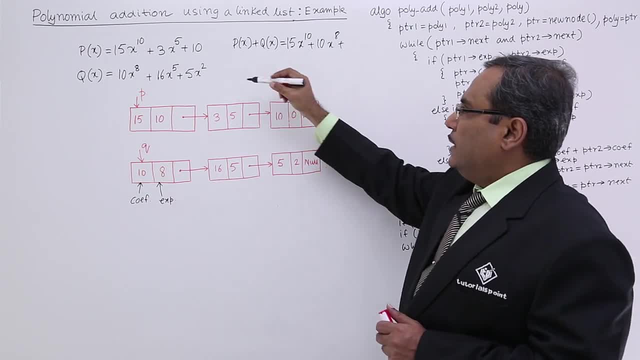 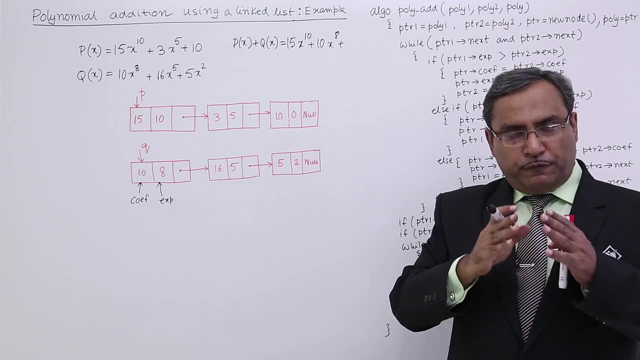 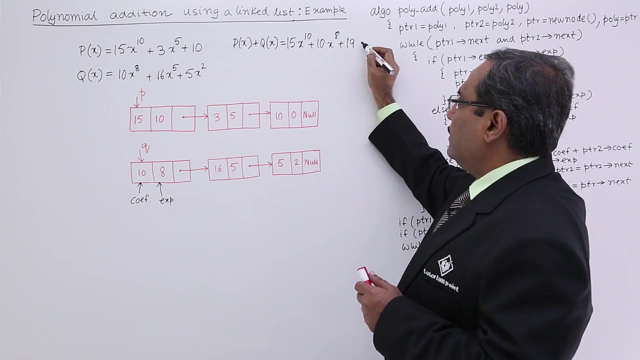 them. So 10 x to the power of 8.. Here you see, these two exponents are equal. When two exponents are equal, then they should. the corresponding coefficient should get added. So now it will become 16 plus 3.. So it will become 19 x to the power of 5.. So what is happening At first? 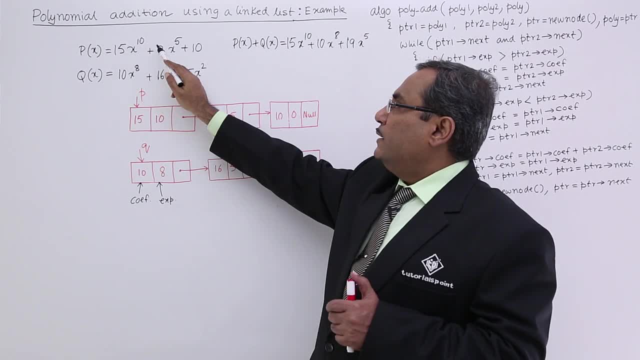 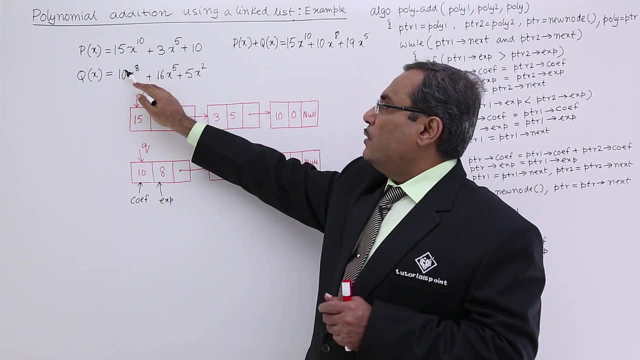 I am copying this one. My observation will be will advance here Now: 5 and 8, 8 is higher, So I have copied this one. So now my observation will be shifted to this. So now I shall compare. 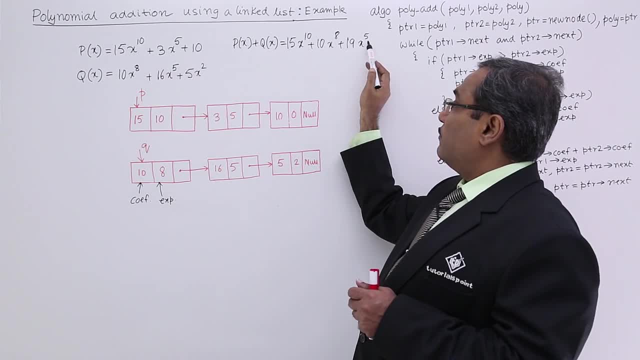 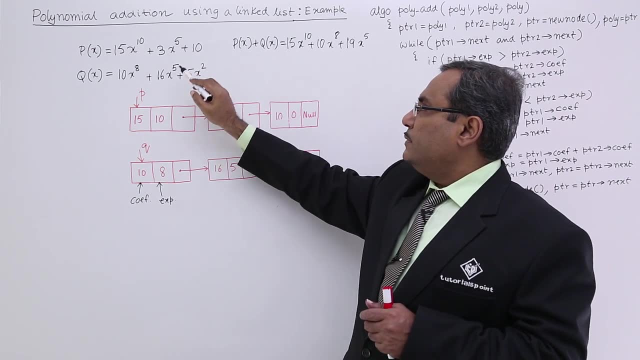 this two, So 5 and 5, they are equal. So x to the power of 5 will come And the respective coefficient will be 16 plus 3.. So 19 will be coming. So my observation will go to this term. 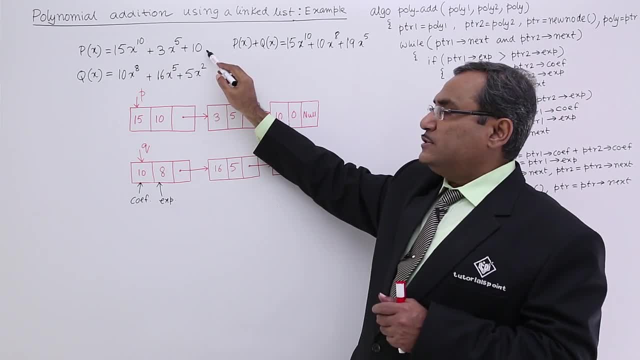 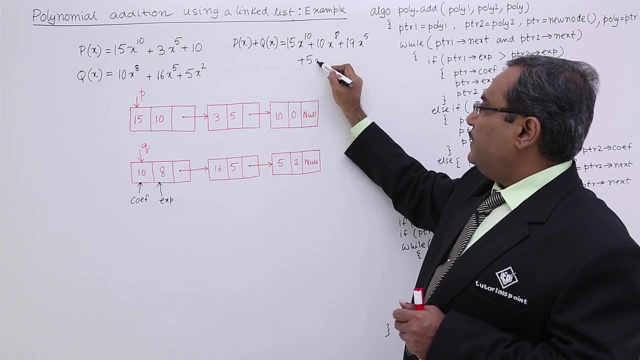 My observation will come to this term. Here we are having x to the power of 0. Here we are having x square, So 2 is higher than 0. So I shall go for 5 x square. So it has. 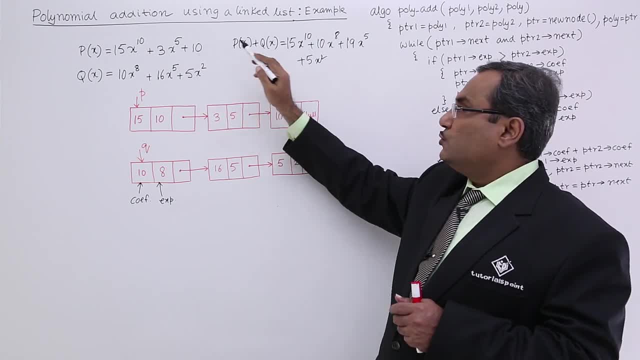 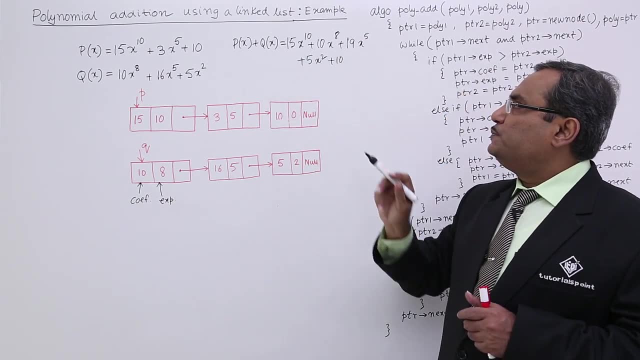 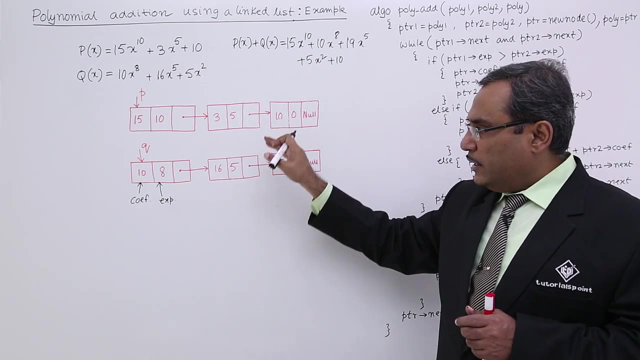 got exhausted, But I am remaining with some terms here. So they will get copied without any comparison. So they will get copied without any comparison. In this way, this p x plus q x will produce the respective results. So we have done it. Now, if I am to do this one, 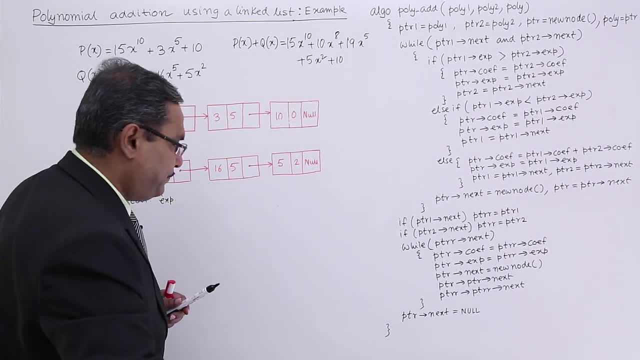 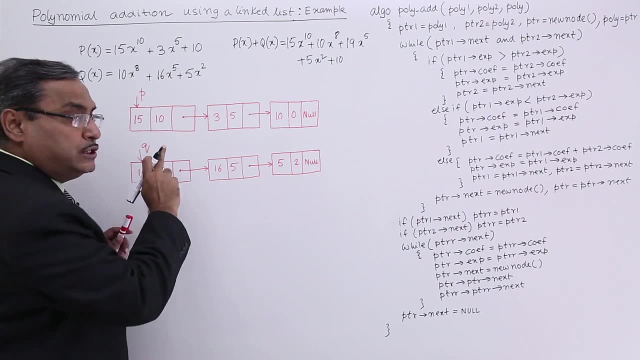 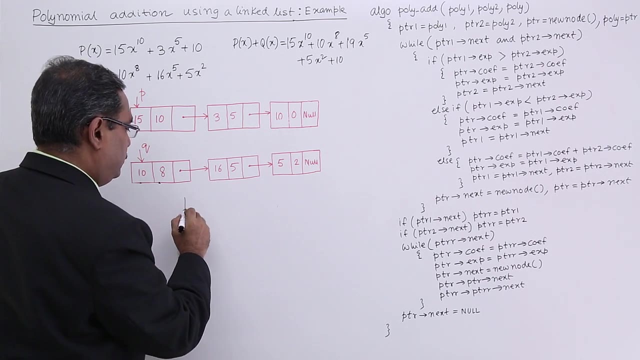 using this linked list, then what will be the scenario in that case? At first, so p and q, they are pointing to this particular nodes. So at first this exponent and this exponent. So 10 is higher, So 10 will get copied. So I am having this 15.. I am having this. 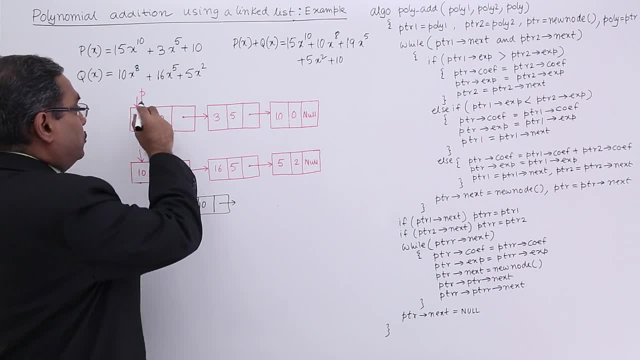 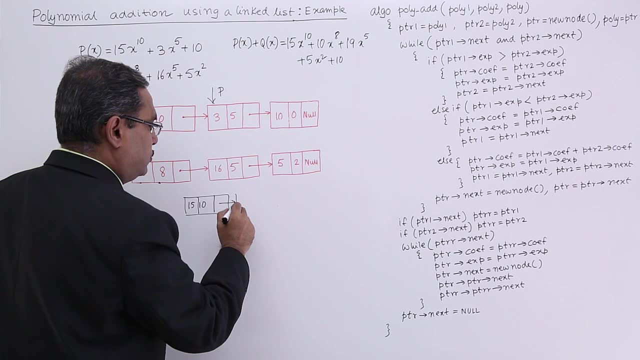 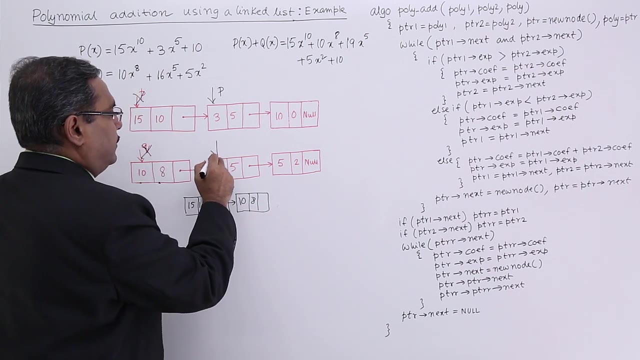 10.. Now it is pointing to the next node Now. so this p will be shifted to this. Now, 5 and 8, 8 is higher, So this node will be copied in the target Link list. So let it be 10 and 8.. So it will be shifted to this. Now these two exponents are: 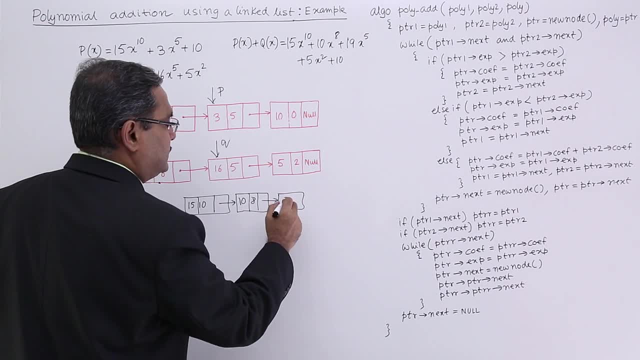 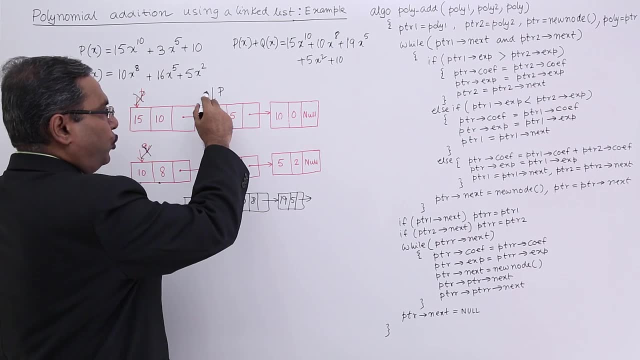 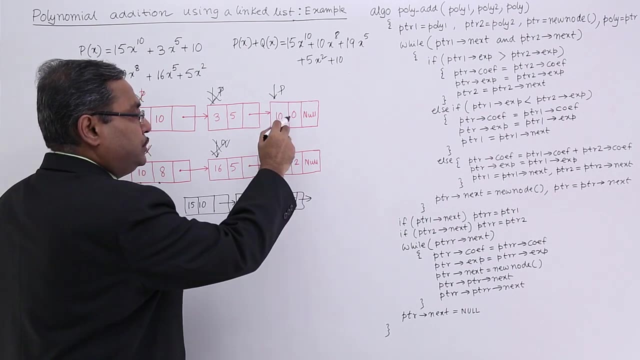 same. So what will happen In that case? this coefficients will get added, Any one of the exponents will get copied And both of them will advance because the respective nodes have got processed. So now 0 and 2,. 2 is higher, So the next node is higher, So the next node is higher. 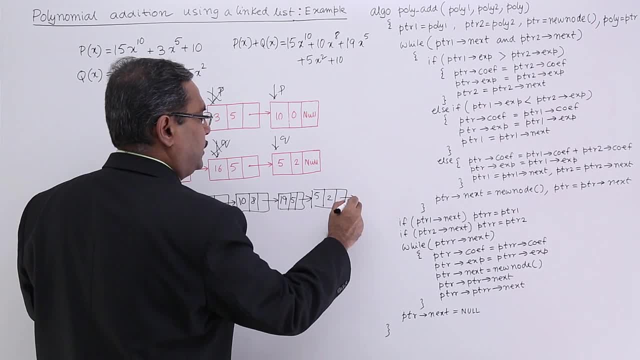 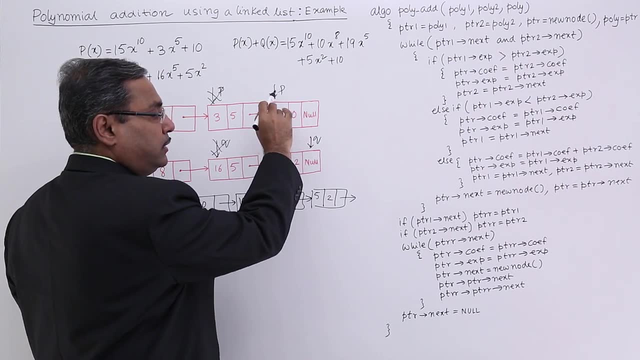 So the next node will be 2.. So 5,, 2, it is pointing to this node. Now it will be pointing to this null. So q has got exhausted, But p is still not null. So it is, whatever the nodes, it. 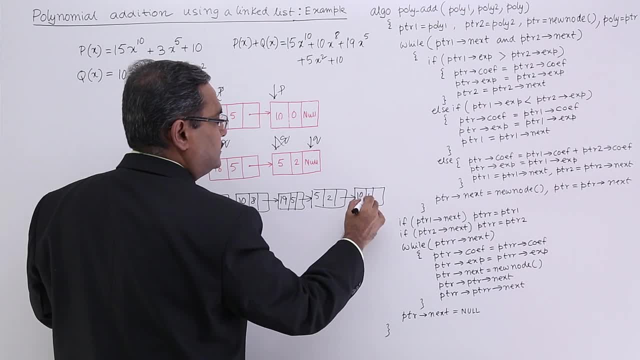 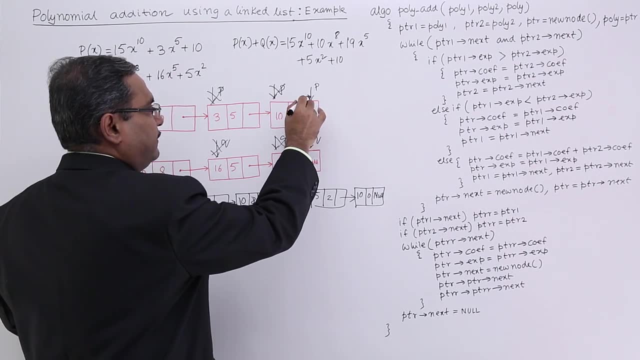 is having. so they will get copied here. So it will be 10,, 0 and null. So p will be advanced to this particular place. So when it is advanced to this particular place, then p and q both are null. 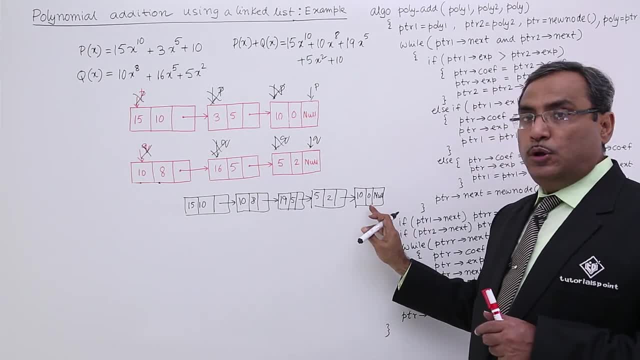 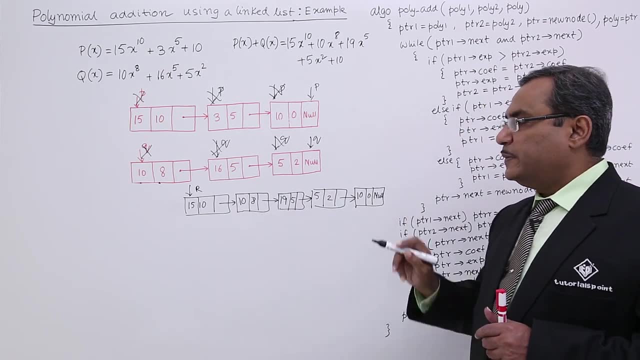 So the algorithm will terminate. So in this way my result will be produced, And here I shall put another result. So I am making this one as r, So r will form this particular linked list. So this is my basic logic, which is: